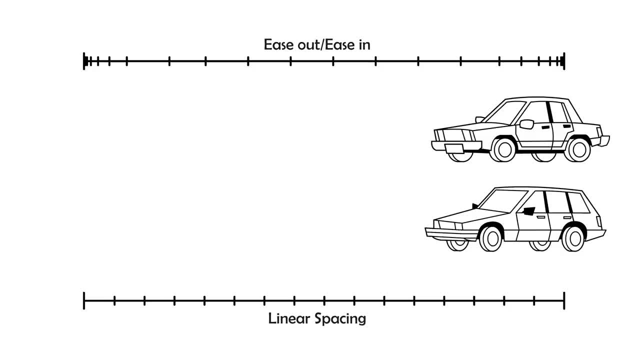 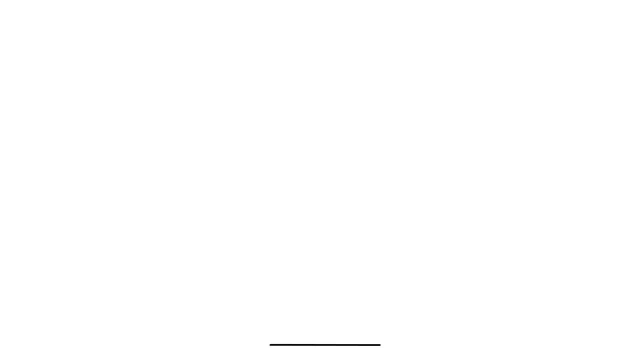 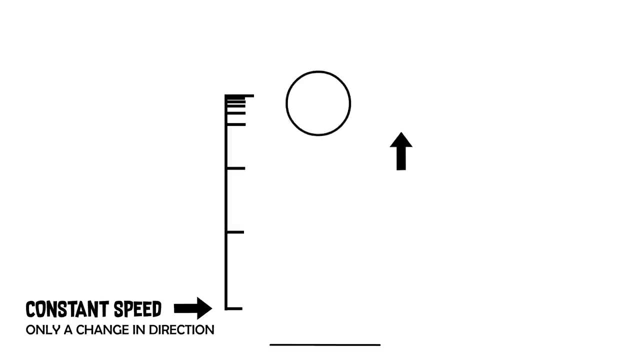 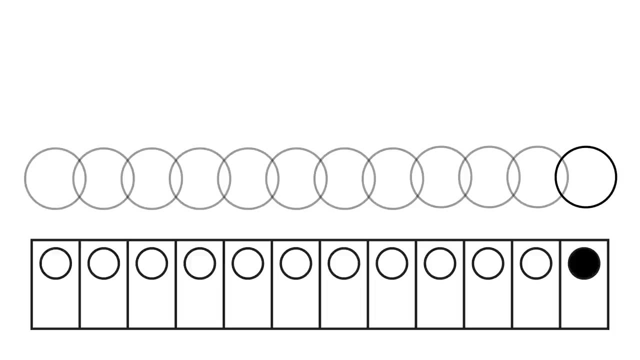 Instead, it maintains its original velocity and shoots back up, And then it can ease again at the top as it loses momentum Because the frame rate of animation is so constant. the way that we achieve easing is by adjusting the spacing between each drawing. 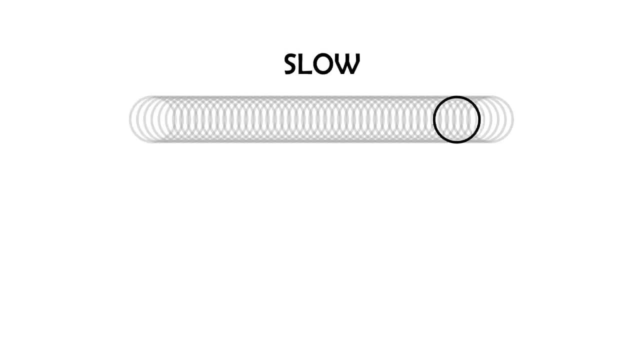 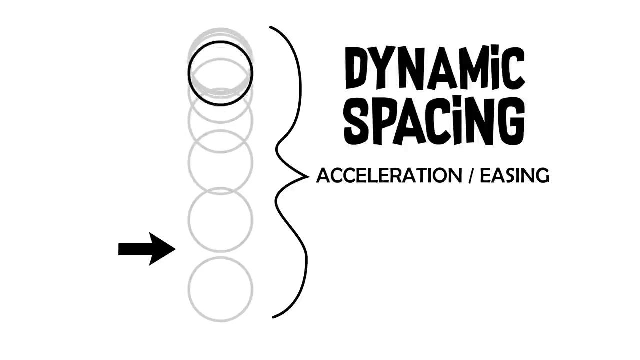 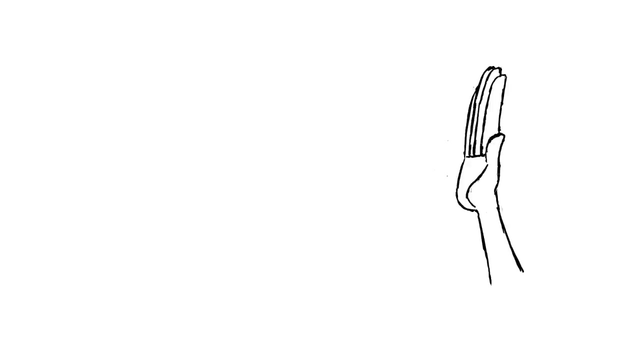 So drawings close together make slow motion, and drawings far apart make fast motion. notice how the drawings at the top here are close together and then become further apart as the ball falls. this is dynamic spacing and this is how you create acceleration or easing. let's try a hand, because we are learning to animate characters, of course, and move. 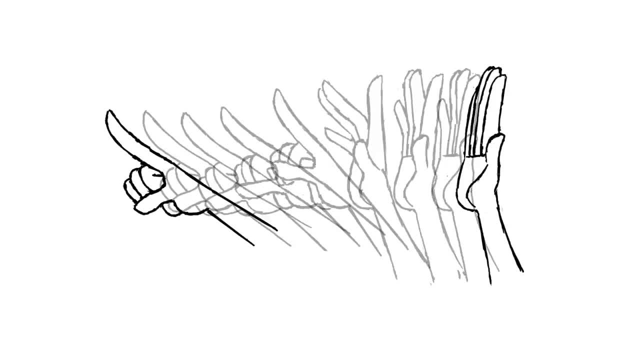 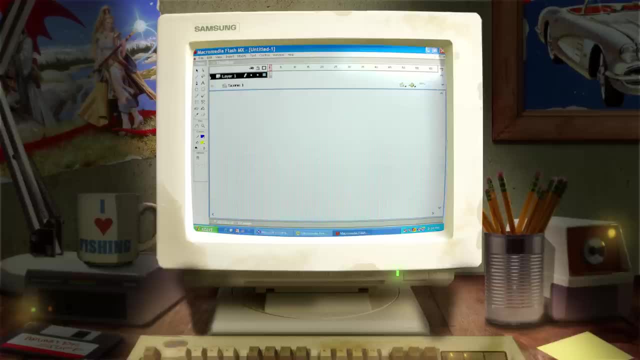 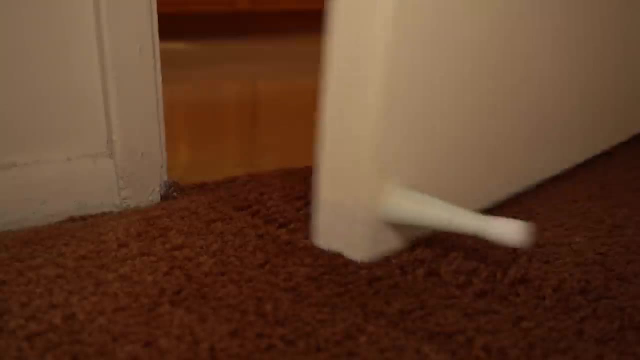 it from A to B, but not like that with easing. okay, that's pretty good, but it could be better. let's add our second principle, overshooting, which is when an object goes past its final resting point only to then snap back into place. this idea might seem overly cartoony, but it can add so much life to your characters. 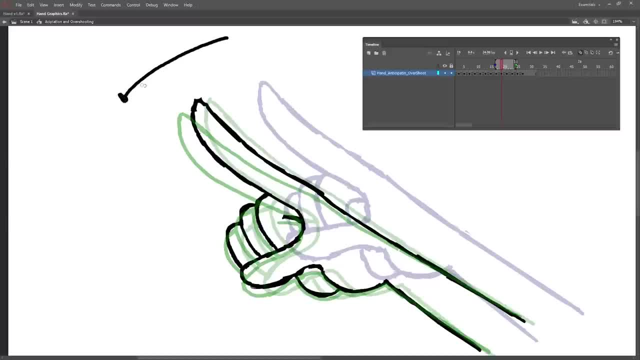 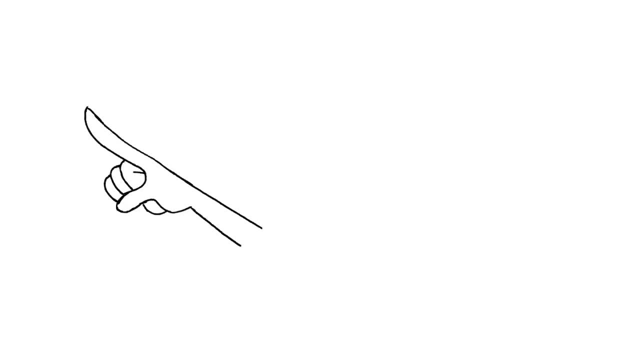 movements. I'm gonna adjust the final frames to go past for two frames. then it will move back here and then go a little bit forward and then finally settle. okay, look at the difference. now you can see how adding overshooting at the ends of your animation brings even more life. I mean, it's not possible unless you're a. 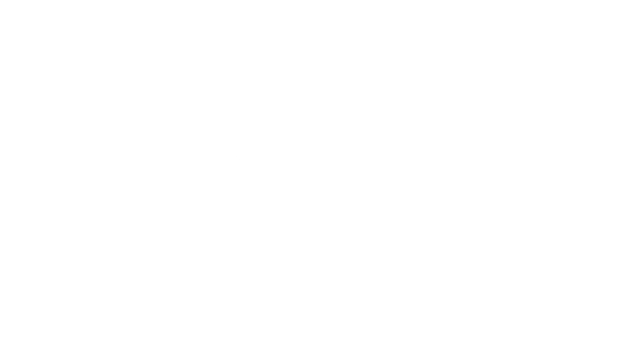 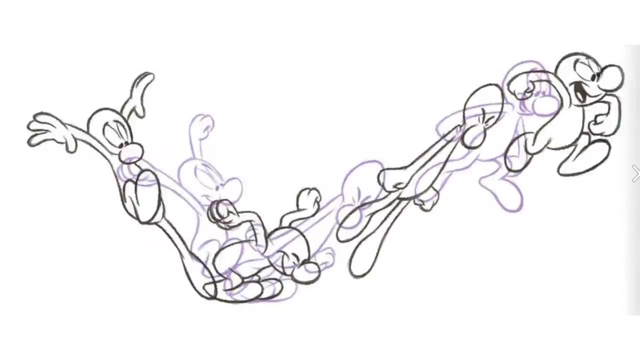 robot to come to a perfect stop. so unless you're going for some crazy stiff warp in, even just adding one frame of overshooting can do so much. characters are organic things and they change shape as they move. an animation should exaggerate that. squash and stretch is a principle that emphasizes elasticity. 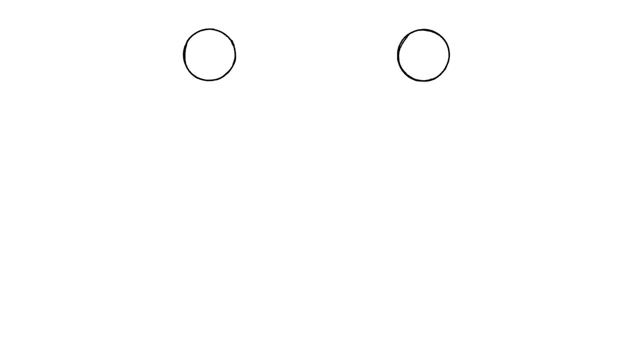 and that's what we're going to talk about in this video. but before we do that, let's show the frame at the beginning. let's look at these two ball bounces on the right. the ball is changing shape. it looks so much more malleable and elastic. 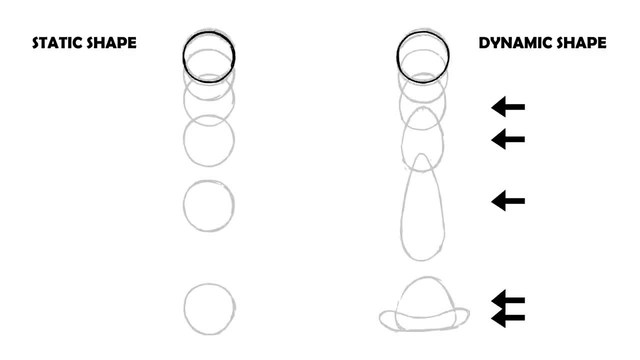 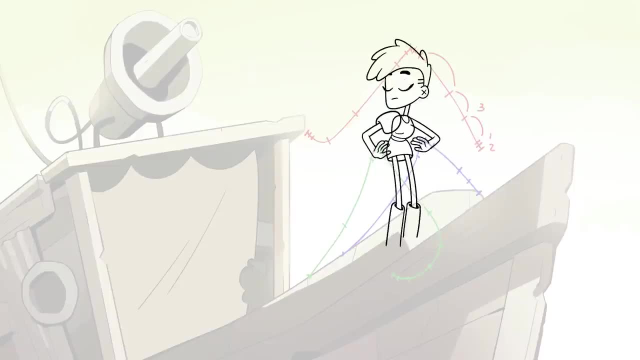 because I changed these frames right here to make it either look squished or stretch. this helps emphasize the movement. might not seem like this is something you should do to characters, but a bit of squash and stretch can go a long way in conveying movement. let's go back to our hand for a second and talk. 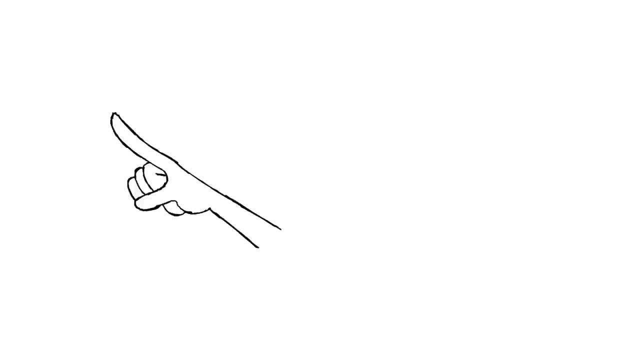 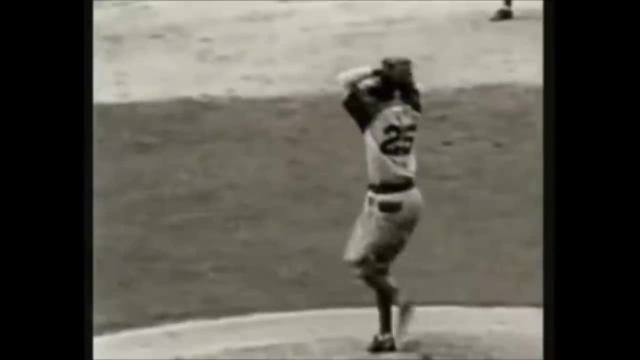 about anticipation. right now, the hand just sort of moves forward. but what if there was a tiny little heavy movement and then the lines moved forward and the little hesitation as if it was getting ready to move forward, sort of like a windup for a pitch? 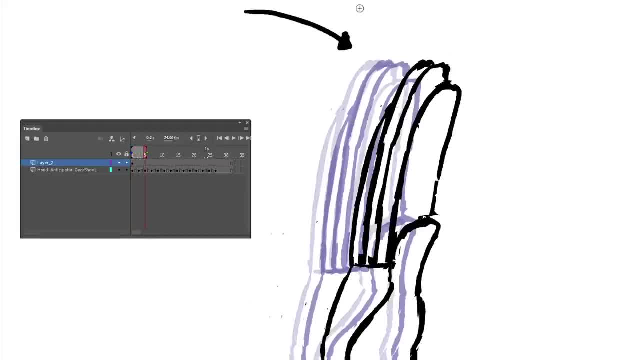 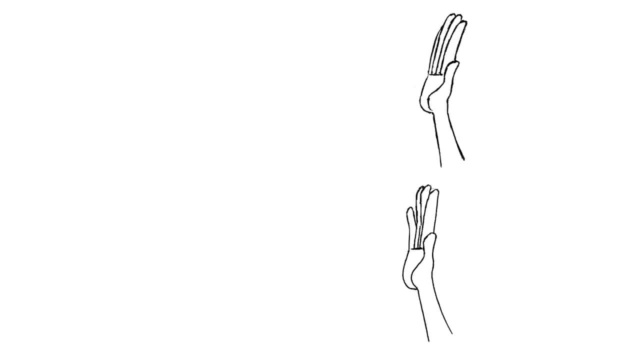 And let's do something more subtle. I'm going to have the hand ease backwards first, right here in these frames, and then speed forward to its final position. Look at the difference. So anticipation is not always natural in every movement, but it is a lot nicer to look at. 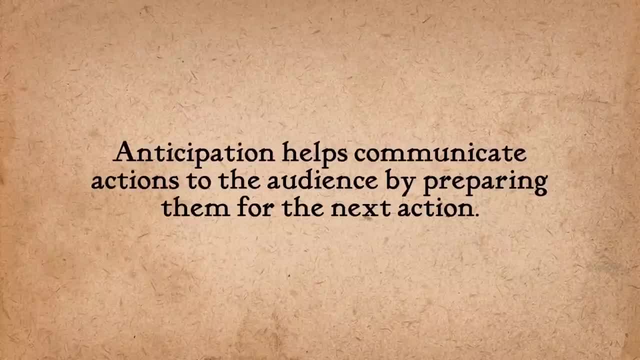 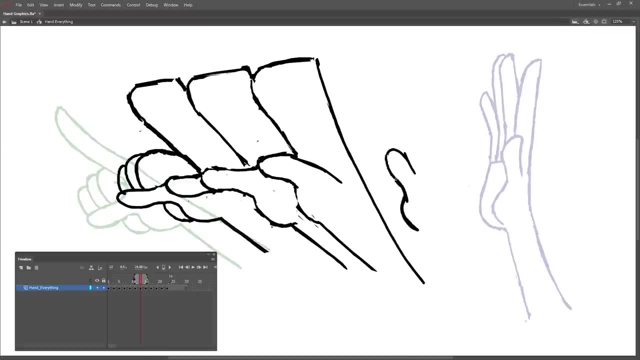 and it makes the acting clear. Just like Alan Becker said, anticipation helps communicate actions to the audience by preparing them for the next action, So they won't miss it. Oh, and I forgot to add in the part where we add squash and stretch to the hand. 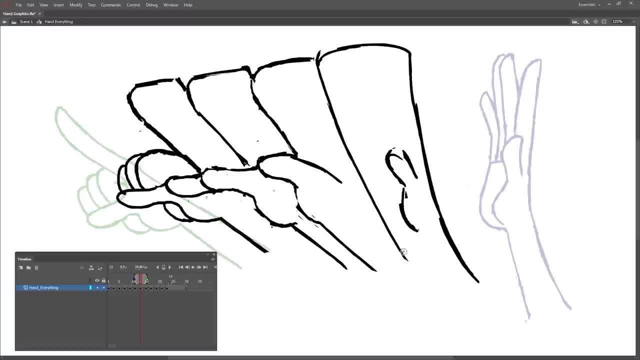 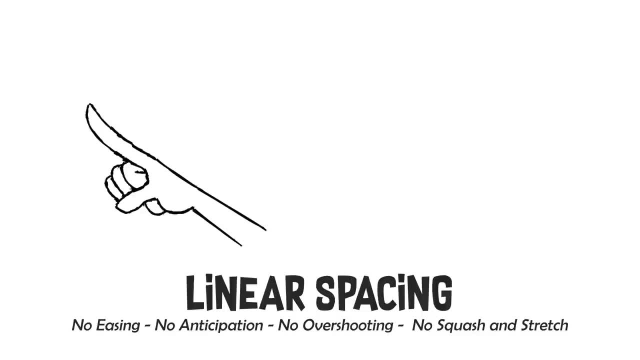 So let me replace some of the middle frames, which are kind of bland, with a very stretchy, smeared drawing of the hand to better convey this speed. Now let's compare the motion of the hand, which uses none of the principles we talked. 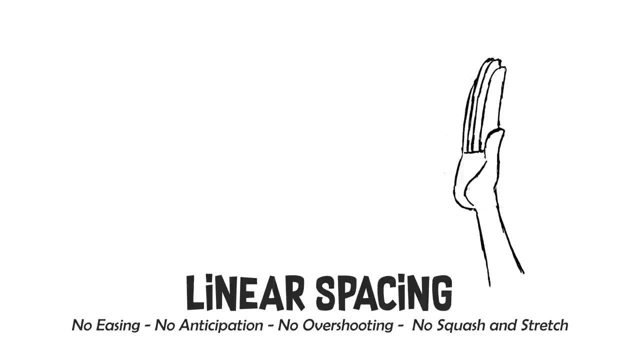 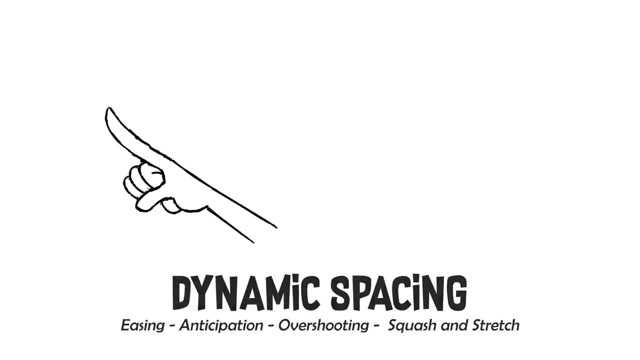 about No easing, no anticipation, no overshading, no squash and stretch. And let's look at the hand where I did everything. Notice the difference. The main difference between bad animation and good animation is that bad animation doesn't move in interesting ways. 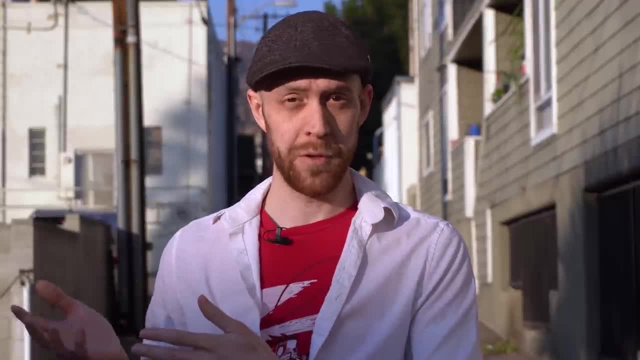 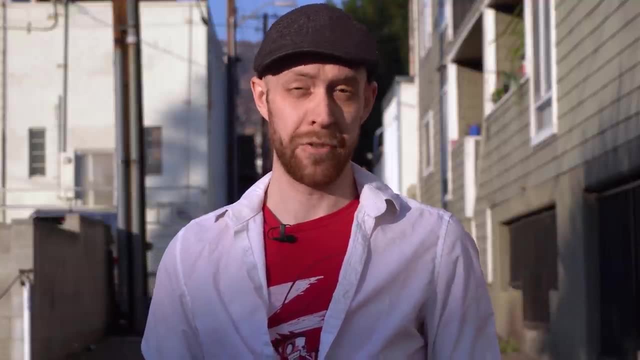 So we know good motion from bad motion, but does that mean everyone who watches this YouTube video can suddenly animate like a 90s Disney animator? Well, no, because you have to train yourself through a series of learning exercises, starting with a ball bounce. 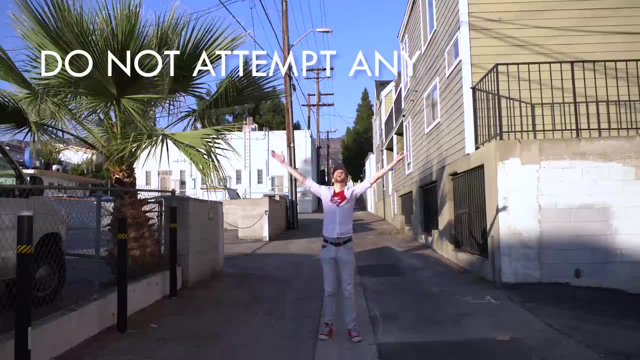 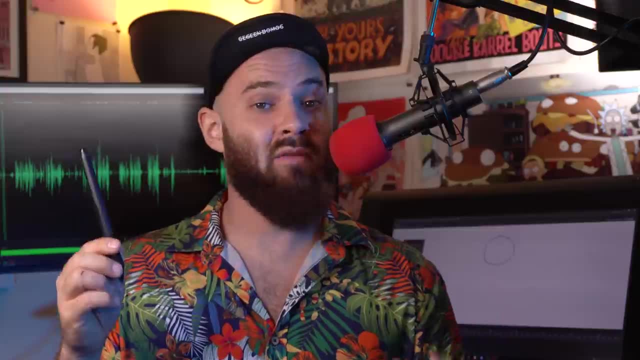 Okay, I don't know if you heard me, but do not attempt any form of animation until you've done a ball bounce. I'm serious And it's harder than it looks, guys. Most people get it wrong because they just open up their animation software. make a ball. 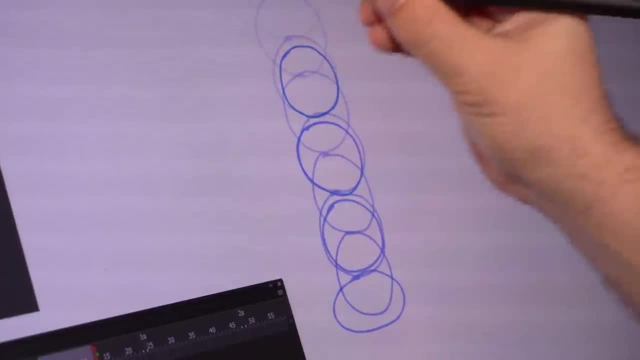 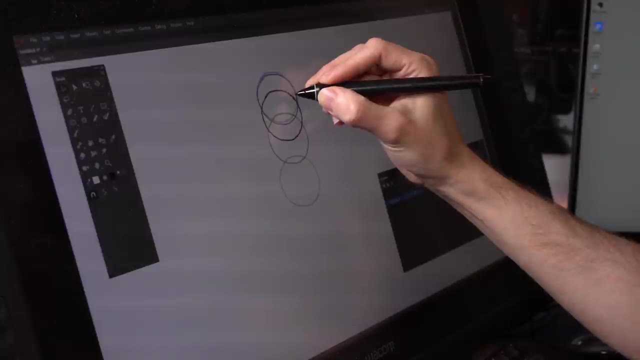 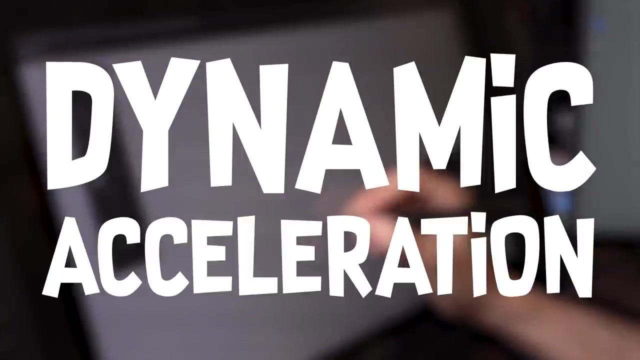 move it down slowly and then back up and say: here I've done it. This looks terrible. There is no gradual spacing at all. Instead, place the top frames really close together and then gradually space them out so that we get dynamic acceleration. 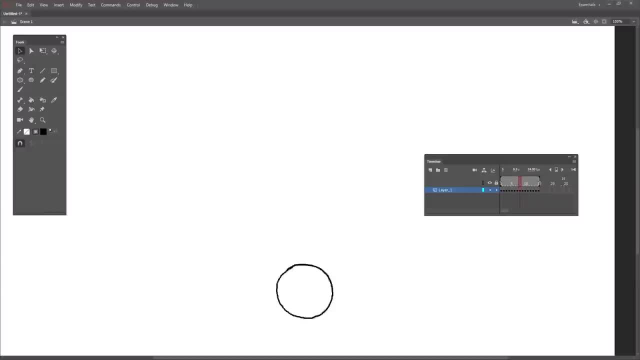 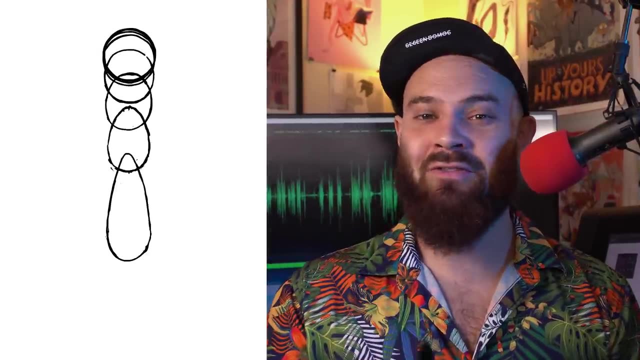 Then you can just copy and reverse the frames until you get your first ball bounce. That is the basic ball bounce, But you can make it interesting By adding a little squash and stretch here and an impact frame here, And if you can do this you'll be strong enough to tackle other assignments. 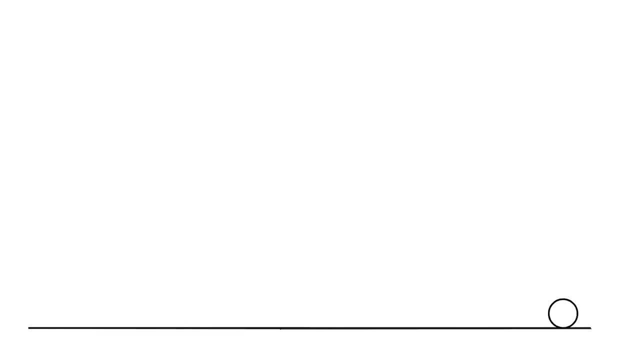 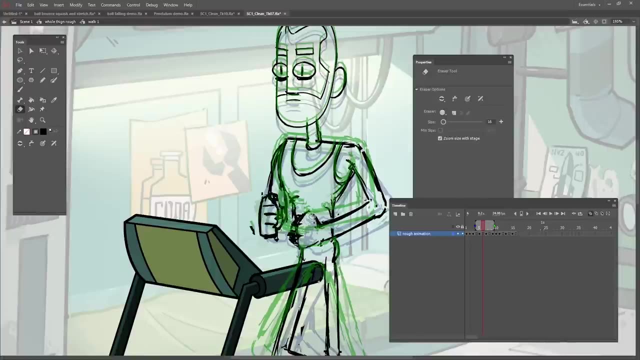 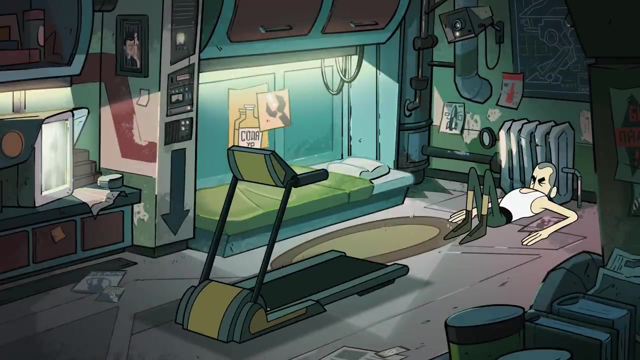 A pendulum, a ball falling, a hand grabbing, a face turning and, in time, build up to a walk cycle. Learning to tackle simple movements will hone your eyes and prepare you for complex, multi-layered character movements. Haven sent us this cat via email. 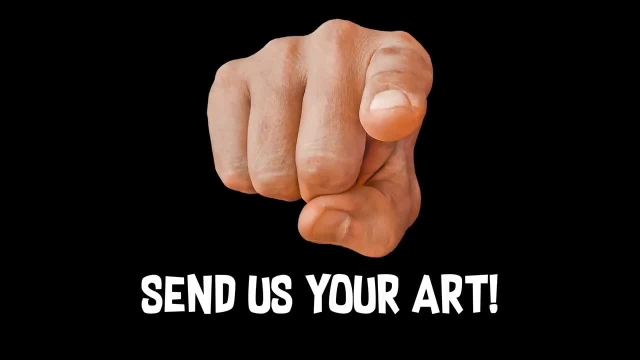 bamredrawmyart at gmailcom. And here it is, And you can send us your drawings too. But now we're going to get him ready for animation. This cat is a little bit 80s with the 3D glasses and the colorful shoes. 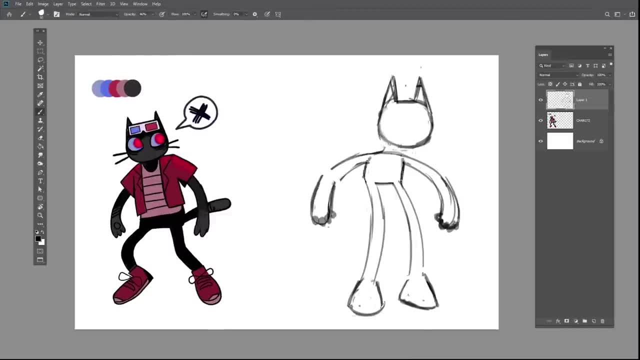 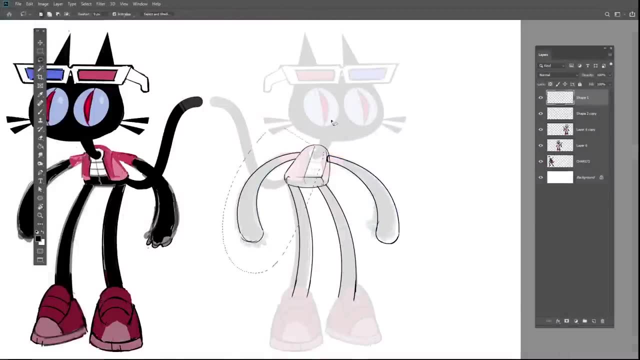 So I just wanted to push these characters' proportions a little bit and use a lot of big round shapes. It's a classic look that you see in Mickey Felix, Garfield and Sonic. Round shapes are very appealing And it's easier to animate something with organic shapes rather than something that's 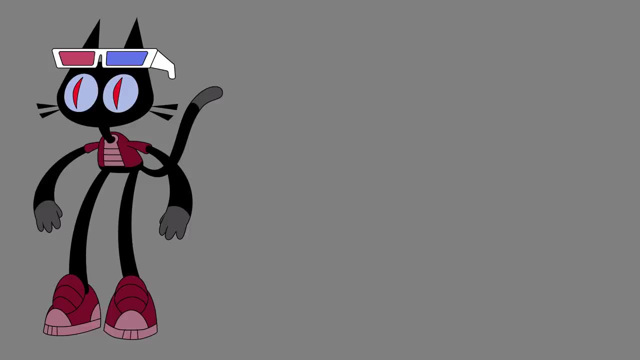 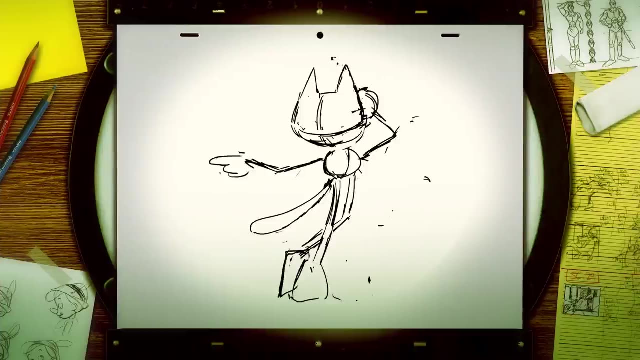 super rigid. Now let's do a turnaround and give it to Brent so that we can start animating. When I'm animating a complex character like this, I want to make sure that I'm doing it right. When I'm animating a complex character like this, I always start with a stick figure. 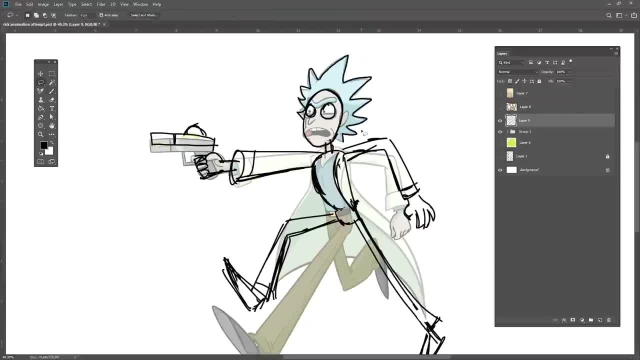 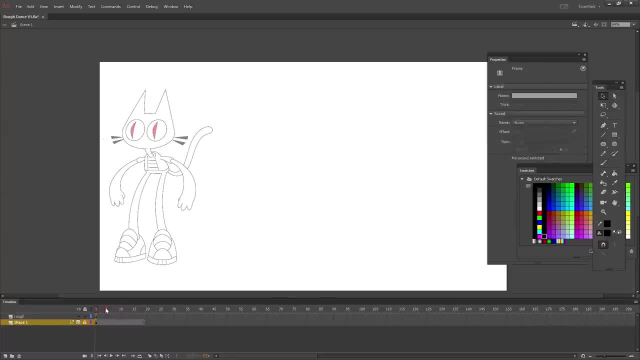 The biggest mistake new animators make is trying to draw a complete, perfect drawing of the character and then try to make that really complex drawing move. It's way easier to start with a very simple rough figure that has roughly the same proportions as your character. 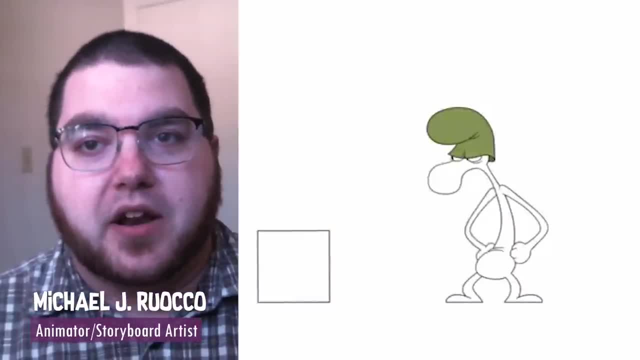 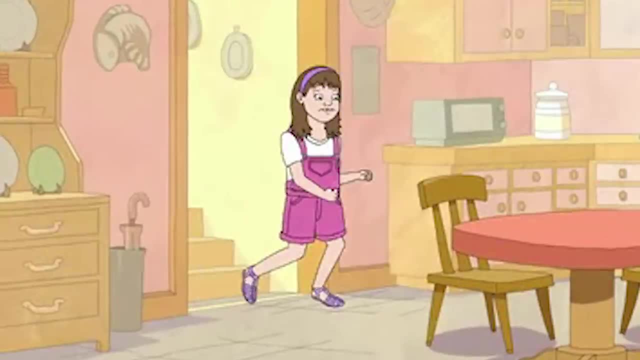 When I was animating Sarah Lynn in the opening of Bojack Horseman- That's professional animator, Mike Rocco- I was really struggling animating her running down this flight of stairs And after several attempts I realized that I was doing it wrong. 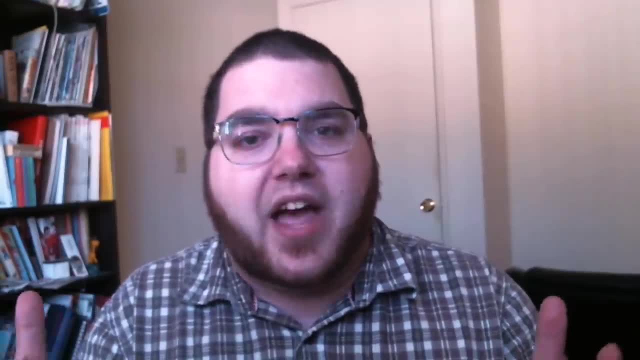 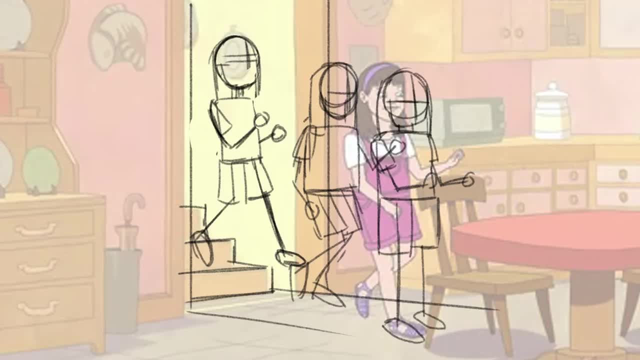 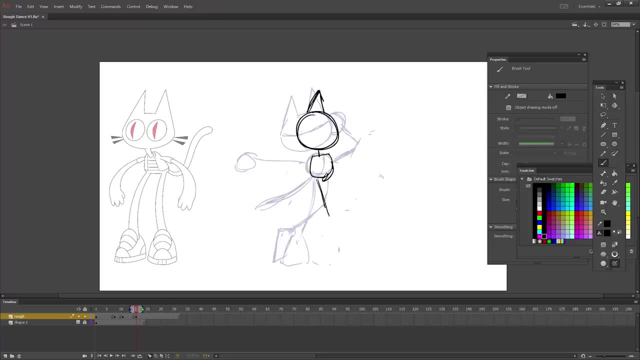 And then I could just animate the final rigged puppet over it. I want him to do a bit of an 80s pop dance, so I found this clip of Michael Jackson doing a spin point. Just like any other aspect of drawing, it's important to have reference for your animation. 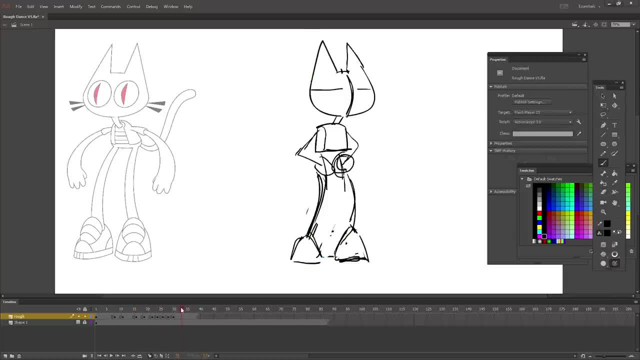 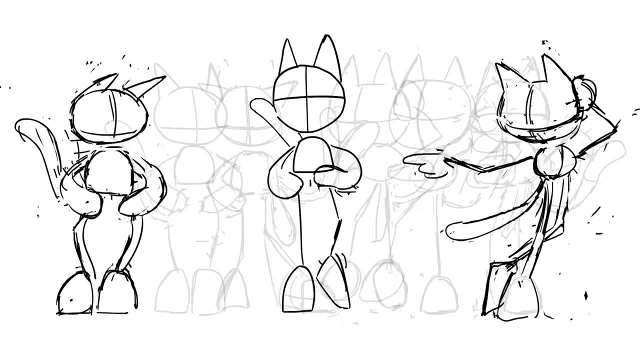 Just in this case, we are not referencing the images themselves, but the movement. I like this motion right here, so I started with that. Then I added a few more actions, connected them with a few breakdown drawings, adjusting the timeline as I went Within a few. 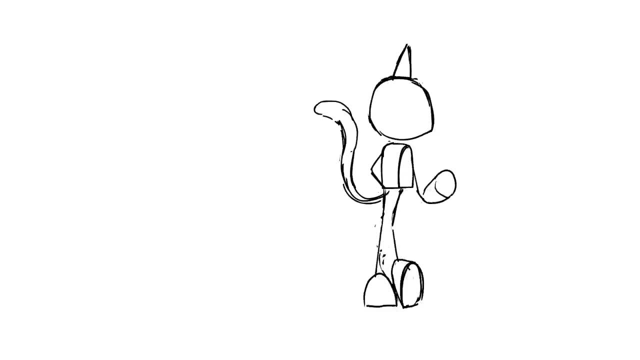 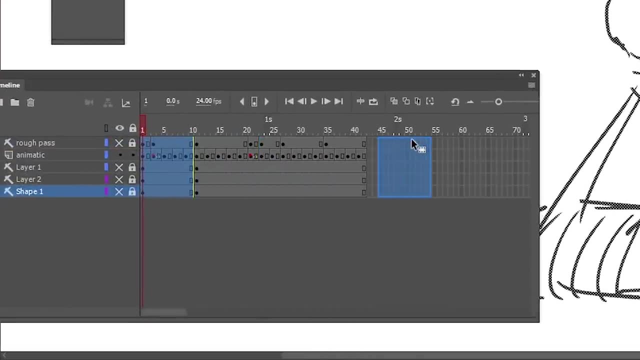 hours I had this rough, sticky looking cat, Even though it's rough. this blueprint will be my guide for the rest of the animation. To get your animation to loop properly, move the beginning frames over to the end, Then you can work directly on the seam. I don't usually rough things out with 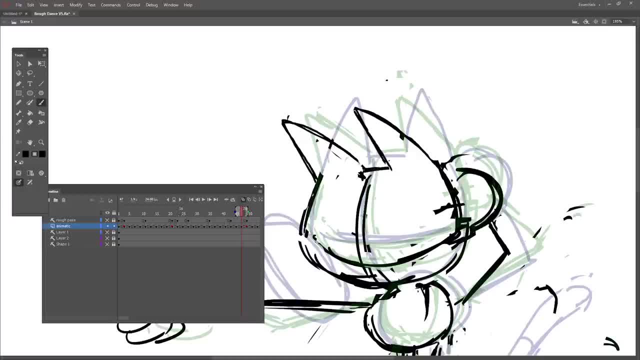 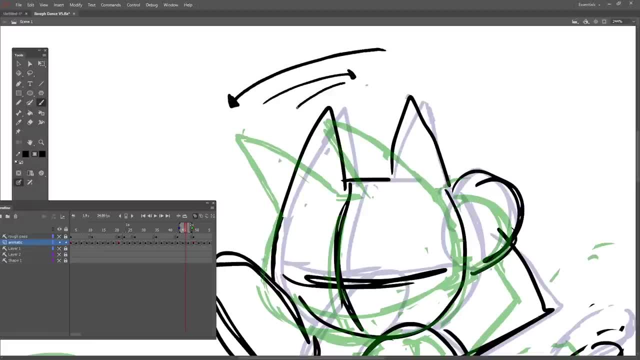 perfect overshooting and easing at first, but once I get an animated stick figure going I can go back in and add better spacing so the motion eases correctly. Right here I can add some secondary bouncing to the ears by adjusting these few frames. Adding little touches like this is very 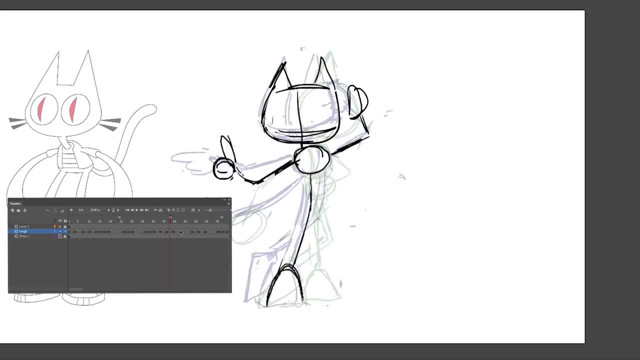 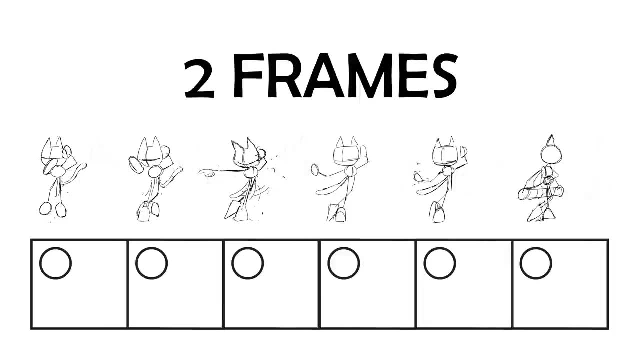 easy at this stage in the animation. As I was working, I added more drawings until everything was eventually on twos. On twos means that each drawing is held for two frames, so instead of 24 drawings per second, you only have to do 12.. Factually, it is much easier to animate this. 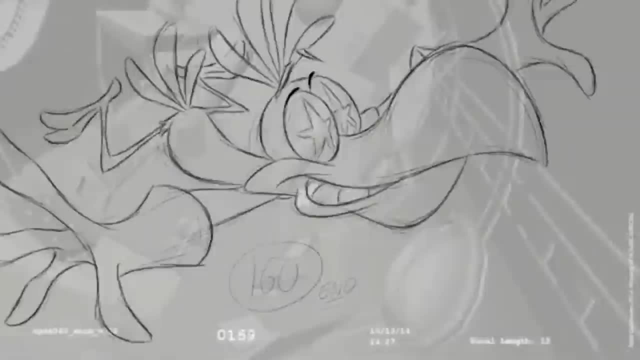 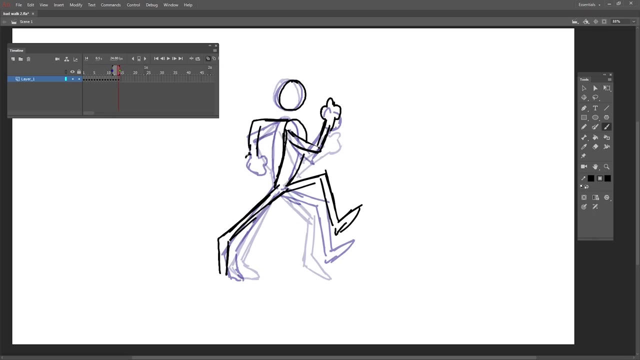 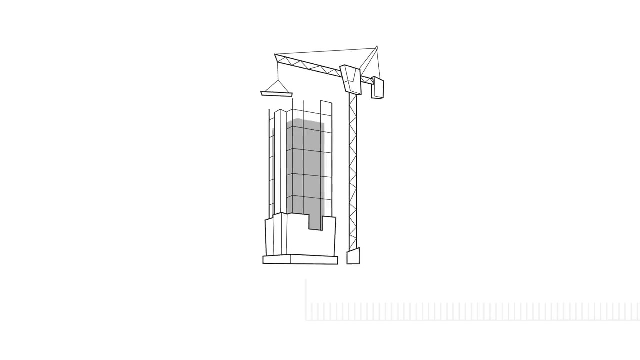 and, subjectively, I think it may be a little bit easier to animate. In animation, you don't really want to clean up the drawings in order, because you can easily end up with a series of drawings that break down over time and end up moving in the wrong direction. Instead, you want to establish a framework for your animation by 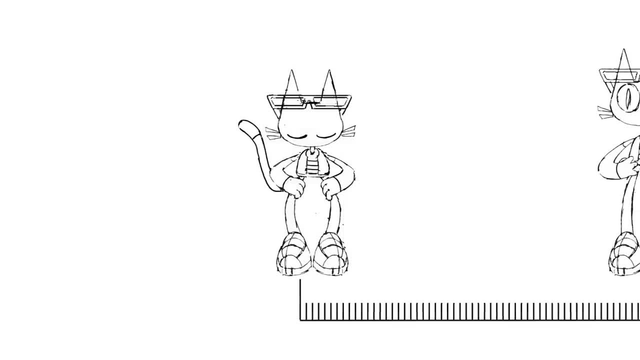 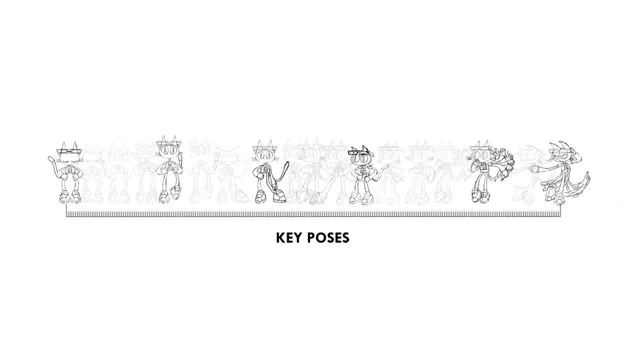 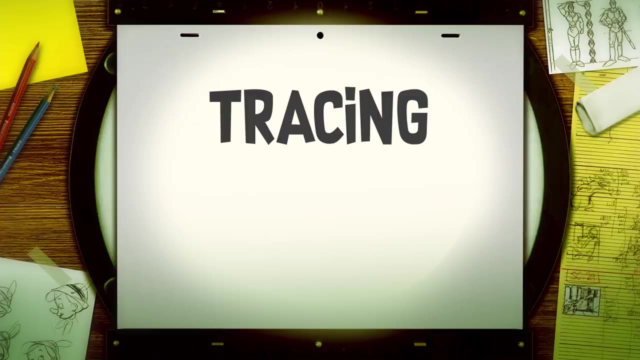 clearly defining key poses that will act as load-bearing drawings to which the rest of your drawings will be attached to. I chose the strongest and most defining poses, and I want these to be the best drawings. The secret to animation is tracing the model sheet. 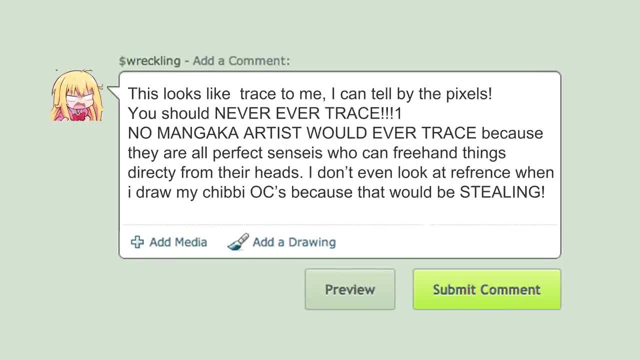 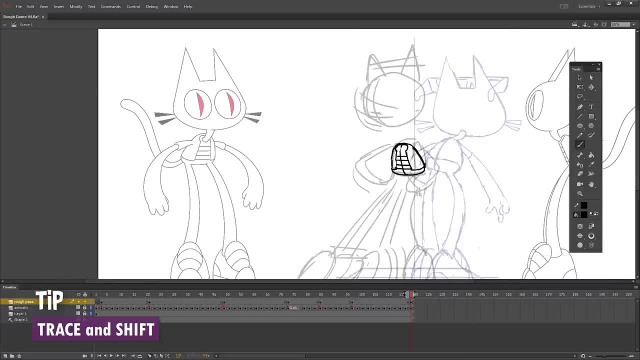 I know that people on the internet have told you that tracing is bad, but in animation, tracing is a very useful tool. Animators do something called trace and shift In order to get my key poses on model. I would sometimes start by tracing. 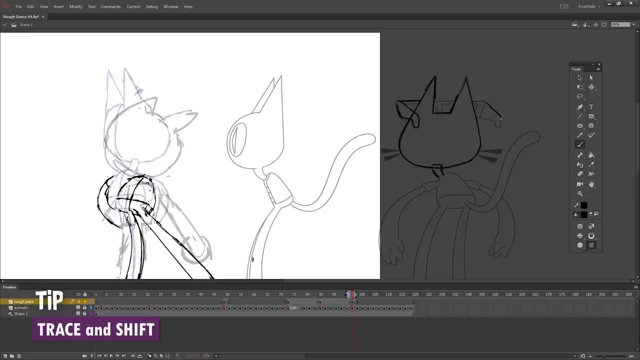 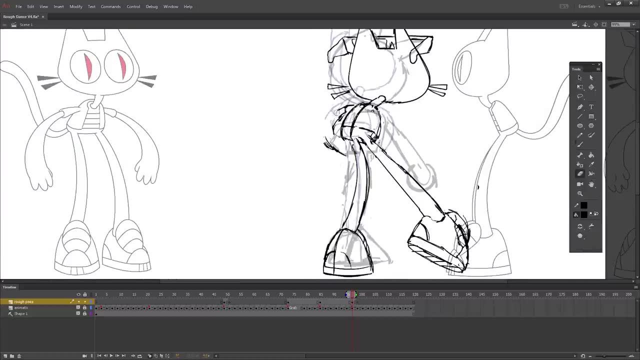 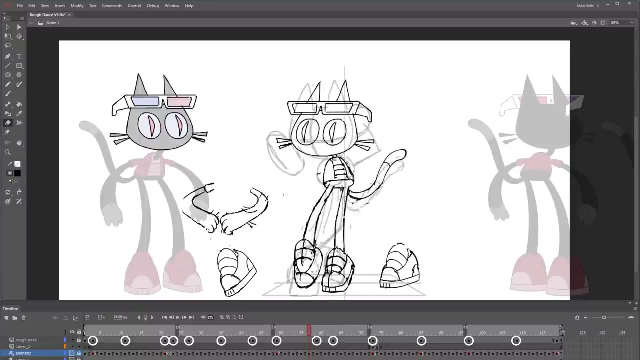 certain elements of a character's turnaround and then shifting them over and adjusting them until they fit the new pose, And so, with a combination of tracing and referencing, this is how I'm able to ensure that the volumes stay consistent. Let's look at where we are now. I have 15 rough key poses timed out and drawn on top of the stick. 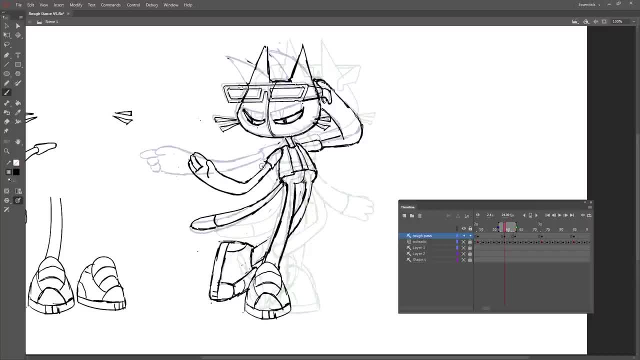 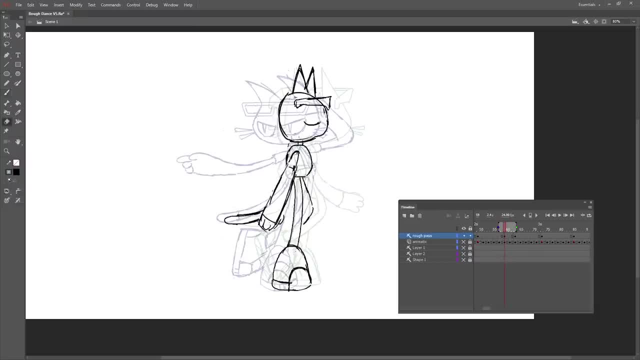 figure animation. Now I can fill in some of the more important in-between poses. These are called breakdown poses and they help define the movement. Notice how I didn't just draw a breakdown pose directly in the center of the two key poses. Remember, most motion has easing to it Like 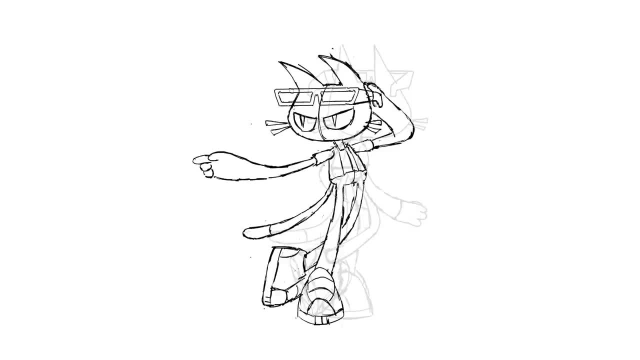 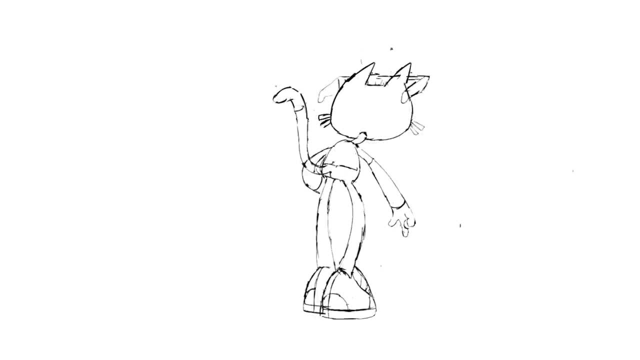 for here, instance, the arm wouldn't just shoot out going at full speed. It's going to do a slow out, but it'll be much closer to the starting position. Also, remember anticipation. Well, it's happening right here. Before he spins around, see how his hand is going back and his foot is coming up. 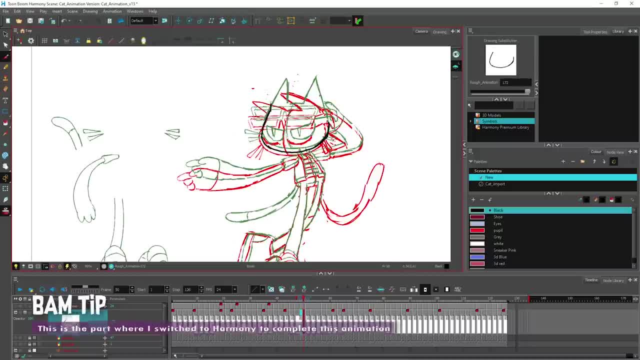 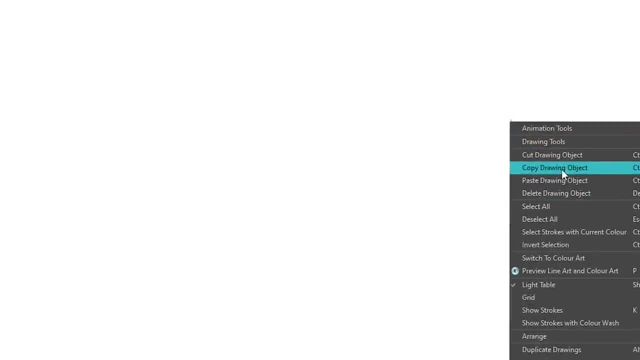 He's winding up for the spin. You don't always have to make every drawing from scratch. Sometimes you can reuse parts of the old drawings by copying those frames and then adjusting only the parts that move, Although I wouldn't recommend overusing this. 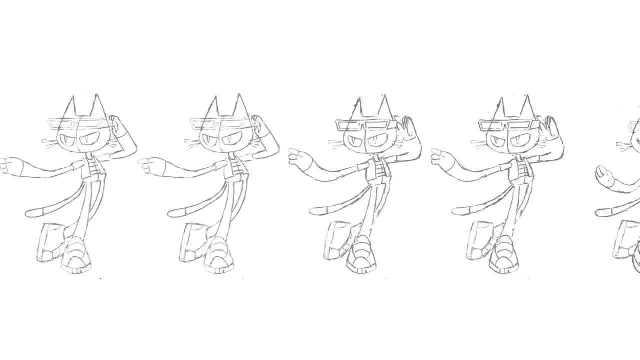 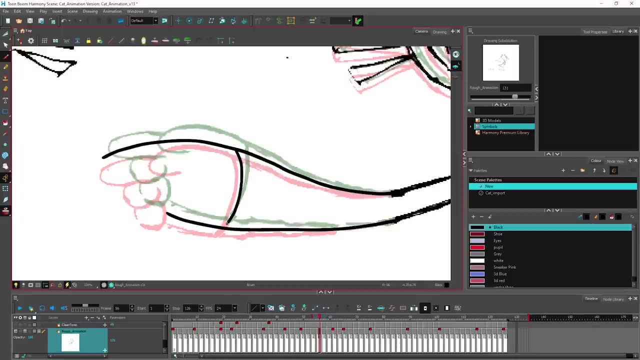 If I have all my breakdowns, I can go back in and do more incremental in-between drawings to smooth out the motion. With onion skinning turned on, I can see where the forms are about to move and I can make a line in between them to build my drawing, Paying extremely close attention to 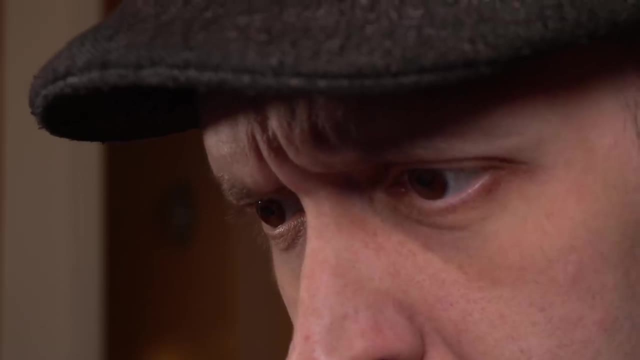 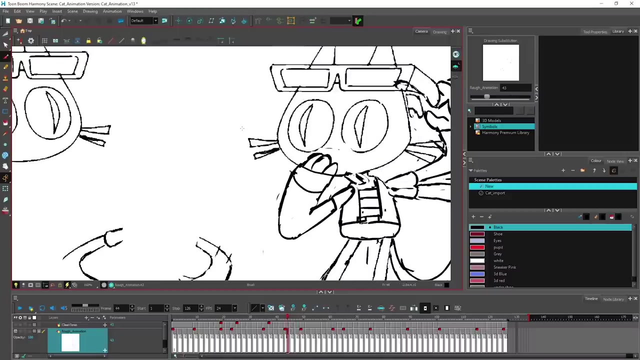 how the forms are moving over time with onion skinning is how you can make your motion look smooth. But you can also just flip, which is just going back and forth between the keys, studying the drawings in motion, If the motion is starting to look choppy, 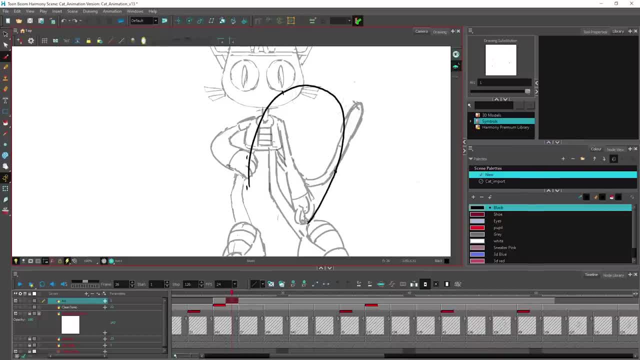 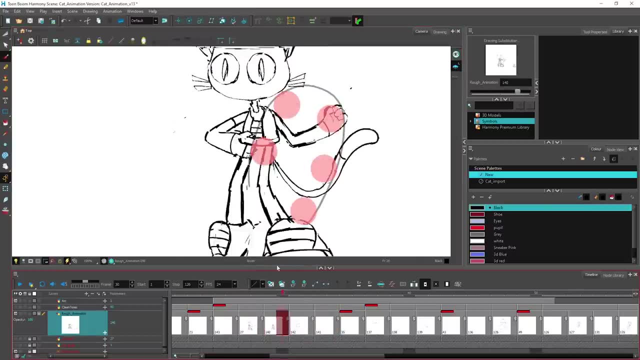 you can draw an arc guide on a separate layer to help you track specific details. Look at this hand. It's moving a bit weird. If we align it to the arc, it's much smoother. Remember overshooting: It's sort of happening in a few places right now. 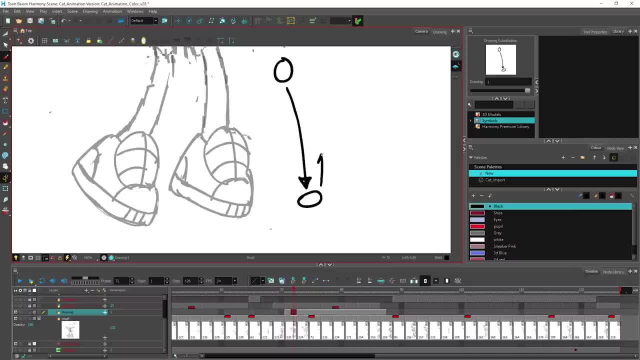 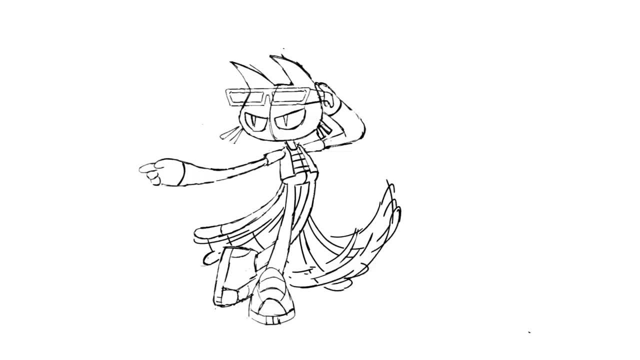 right here on the ears, but also on the feet. When he slams his feet down, I have them getting squashed for one frame and then popping up. There were a few frames that were too fast for the motion to track properly, so I added some. 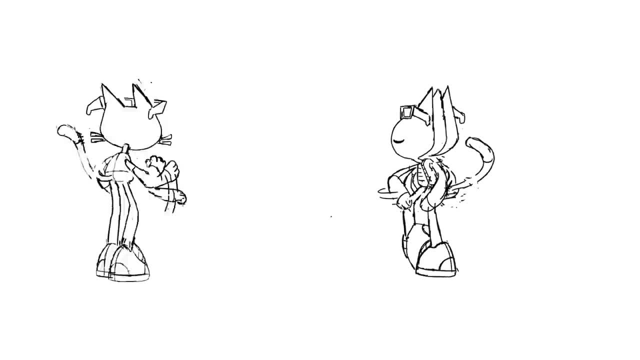 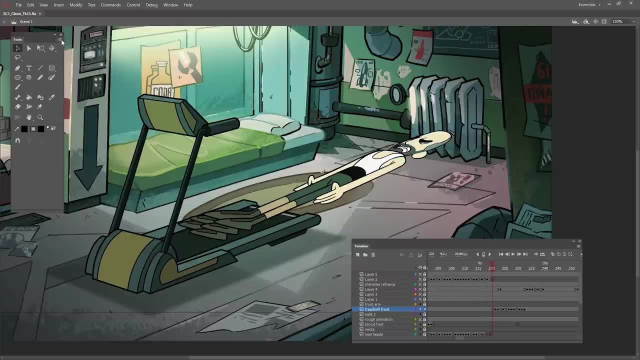 stylistic smears to those frames to make them look a little more smooth. I also added some texture to those frames. Smears are how we convey super fast blurry motion, sort of like how fast things appear blurry on film. A well-placed smear can also add a bit of squash and stretch to your movement. 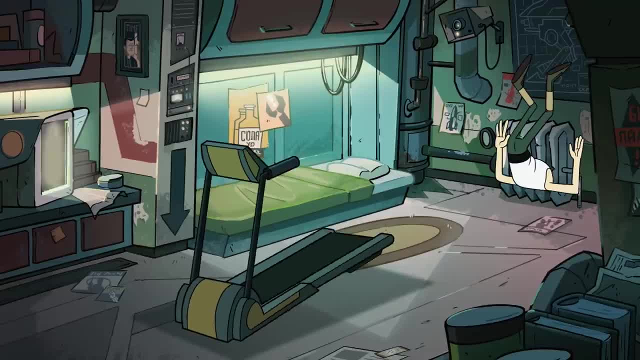 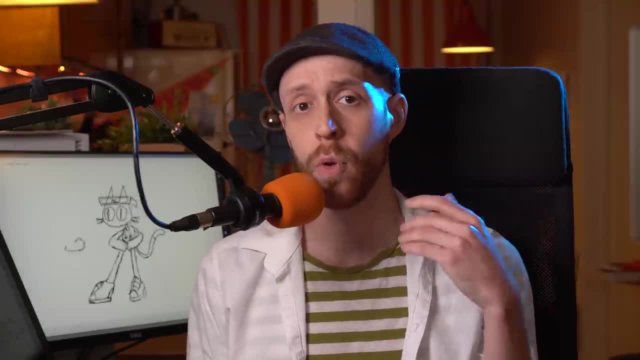 I'd tell you more rules about them, but there really aren't any. As long as your smear matches the motion arcs, it will probably look great. So you do you. Everything I've just showed you was the rough pass which I did on top of the. 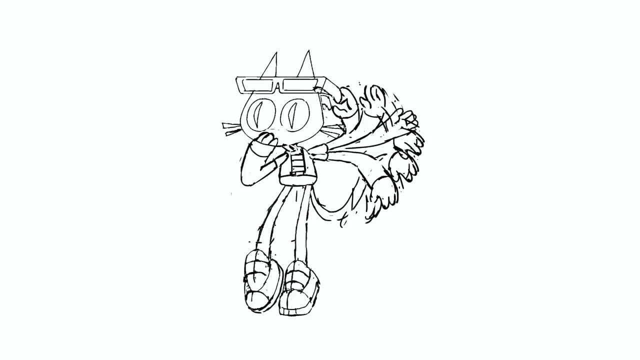 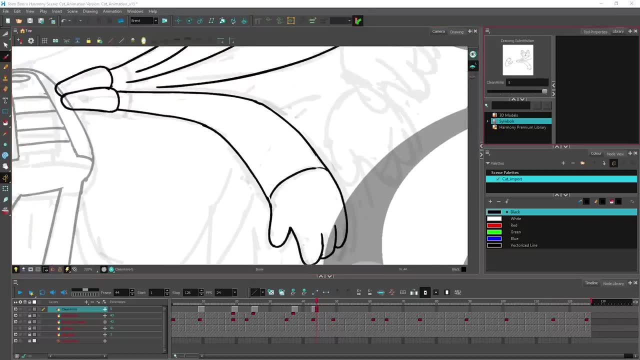 stick figure animation. Now I actually have to go back and clean it up so that it will look clean and it will have color. I wish there was something important I could tell you about cleaning animation, but it's honestly just very tedious. Rough animation can be done fairly. 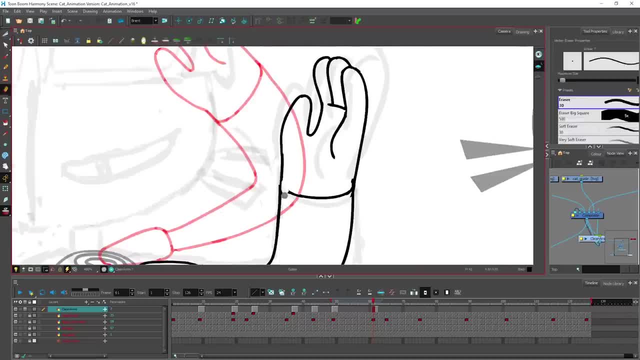 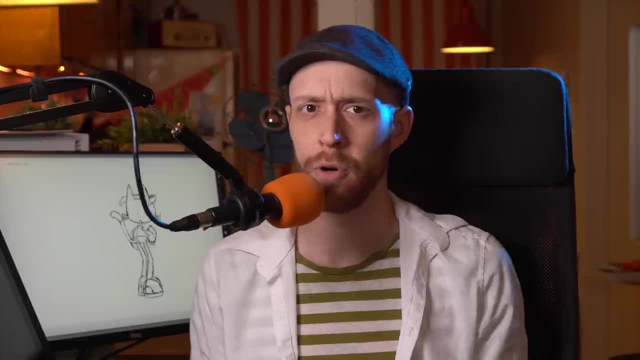 quickly and is forgiving. but clean animation involves triple checking everything to make sure that nothing is out of place and all the drawings are moving together smoothly. I did it in the same order as the rough pass Key poses first, then the breakdowns. 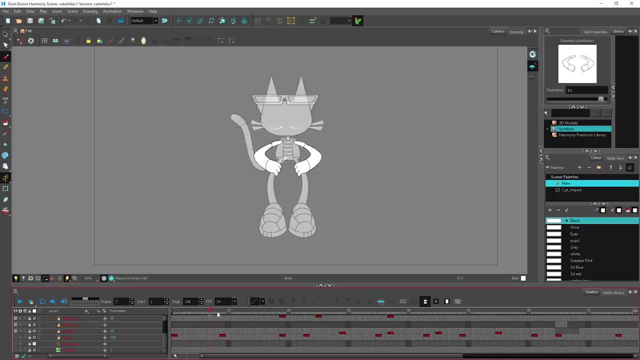 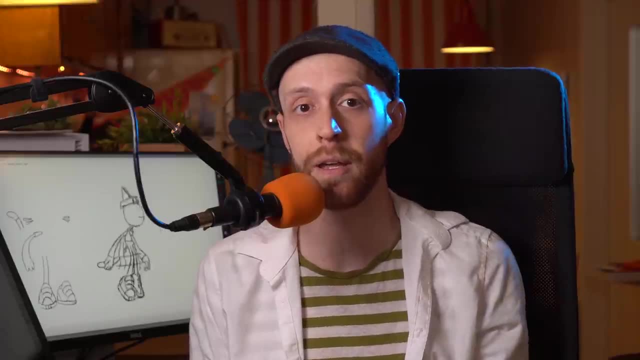 and then the inbetweens. The main difference here is that I did it in layers. The torso, feet and arms are all drawn on separate layers so that if something passed behind the character, I would be able to track it and make sure that the motion was smooth. 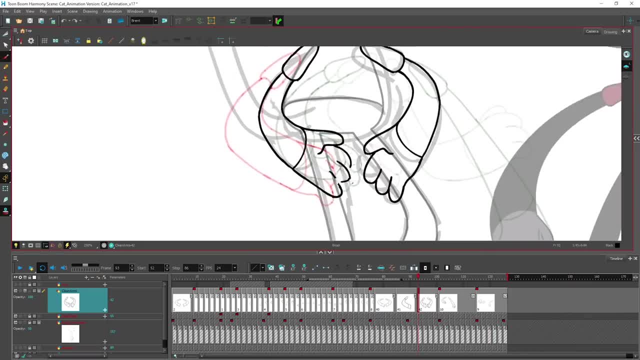 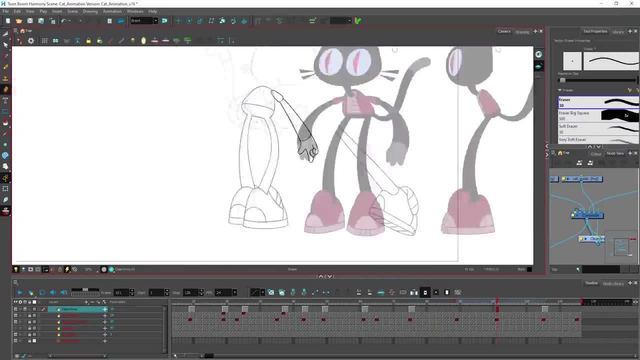 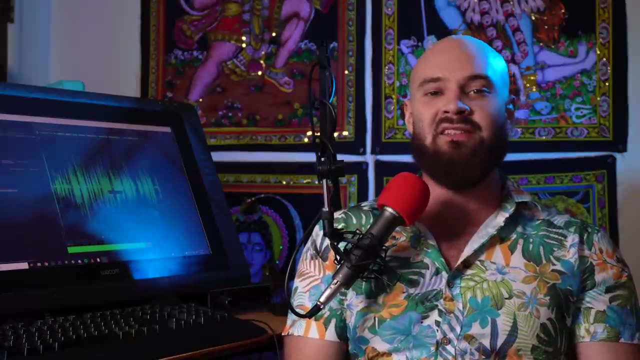 I can't emphasize how long this part actually took. The cleanup was far longer than anything else, and I worked on this animation in my free time for about a year, and most of that was spent on the cleanup. So One question that always pops up is: do you have to color every frame of the animation? 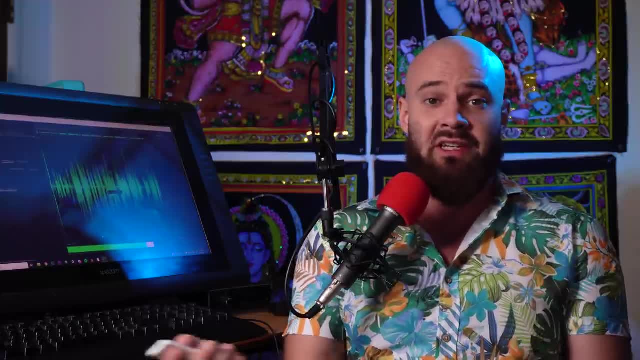 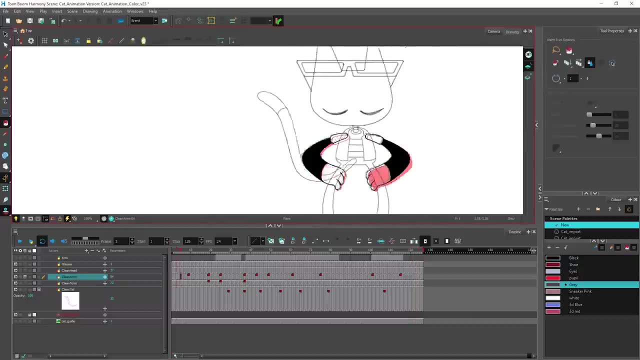 And the answer is yes. Traditionally, you have to color each frame, but the difficulty pales in comparison to actually drawing the animation. I just paint bucket, filled each shape while pressing next frame. Yes, I had to go through every frame, but it maybe took me like a day, whereas the actual animation took. 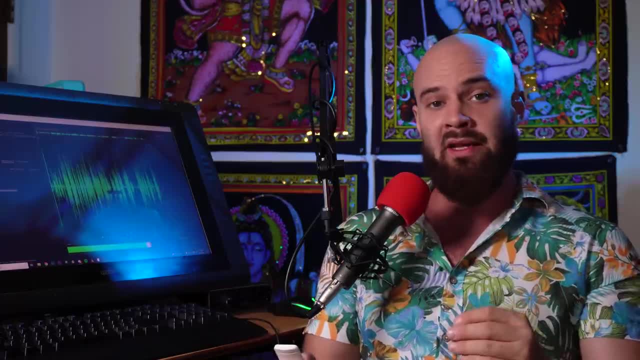 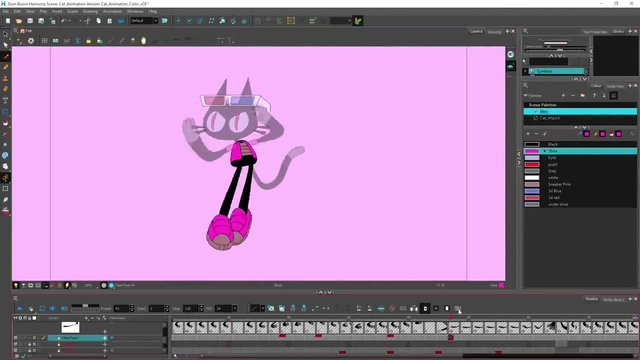 me months, And also you can build palettes in harmony. So if you need to change one specific color, you can do that here and then it will change for all the drawings at once. There are some weird areas that you can't paint bucket fill because the lines don't connect. So